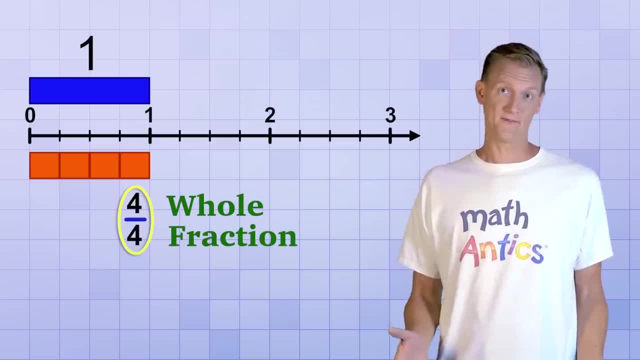 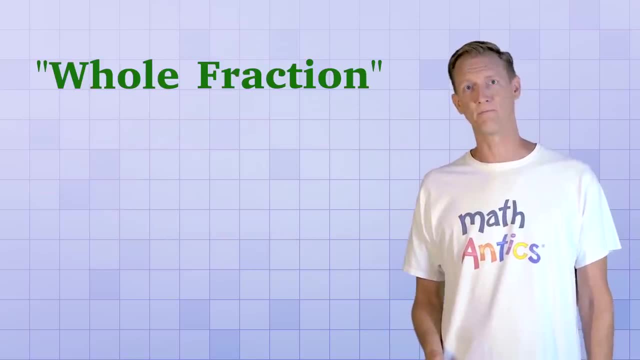 Yep, it's what I like to call a whole fraction, because its value equals one whole. Oh and, by the way, we're going to be using the term whole fraction a lot in this video. It's not an official math term, so your teacher might not use it, but just remember that whenever. 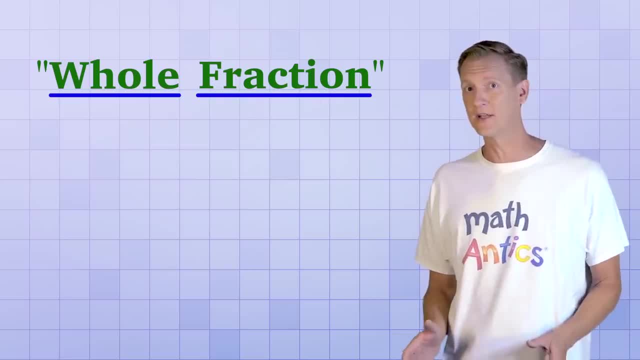 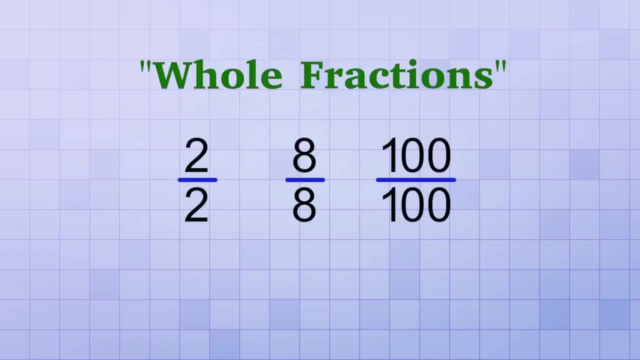 I say whole fraction, I'm talking about any fraction that is equal to 1 whole fraction, Any fraction that has the exact same number on the top and on the bottom- 2 over 2, 8 over 8, 100 over 100, those are all what I call whole fractions. Since all 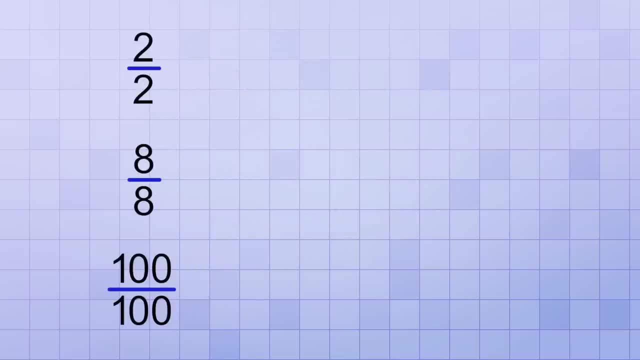 whole fractions equal 1, you can replace any whole fraction with 1.. And you can replace 1 with any whole fraction And you can see how that works on our number line, The 4 fourths all combine to cover the same distance as 1.. 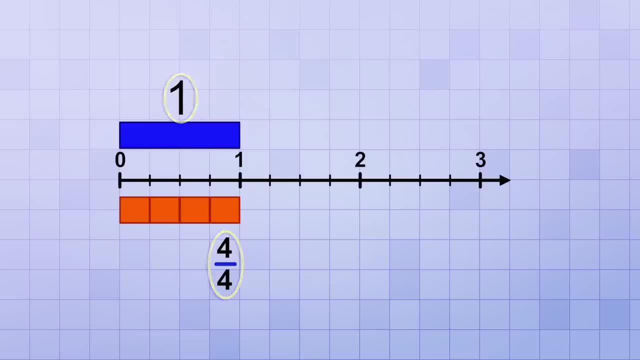 But what if we get a little crazy and add one more fourth? Now we have 5 fourths and we've gone past 1 on the number line. 5 fourths or 5 over 4, is what we call an improper fraction, because the numerator the 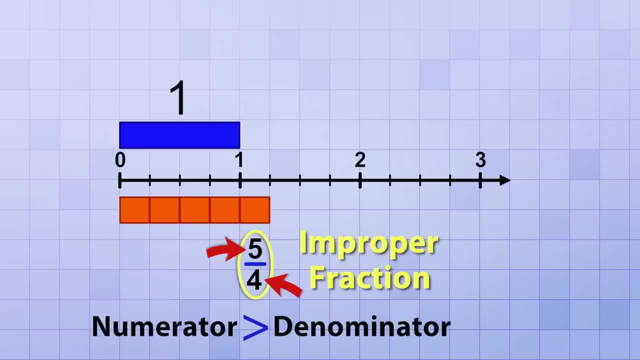 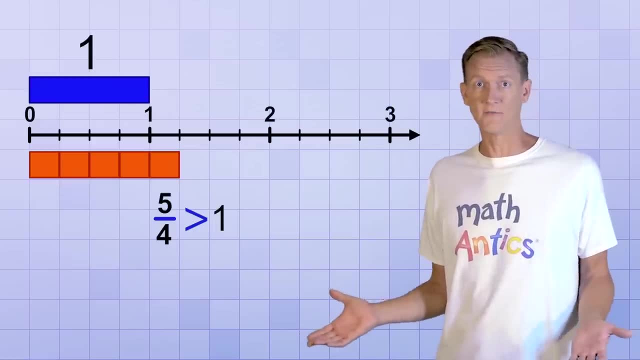 top number is greater than the denominator, the bottom number. That means its value is greater than 1.. In this particular case, how much greater than 1 is it? Well, on the number line, we've gone past 1 by the number line. 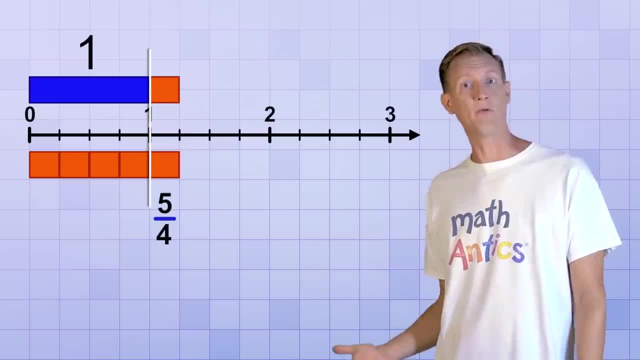 If there is an odd number, we've got 1. And here we have 2,, 3. And we've gone past 1, the fractional amount, 1 fourth. so 5 fourths turns out to be equivalent to 1 and 1 fourth. 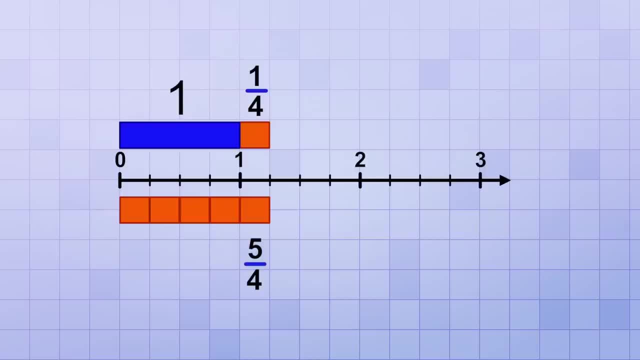 Have a good look at this diagram for a minute, because it shows us something really important about how proper fractions, improper fractions, whole fractions and mixed numbers all relate to each other. First, on this side of the number line, we have 5 fourths, which we know is an improper fraction. 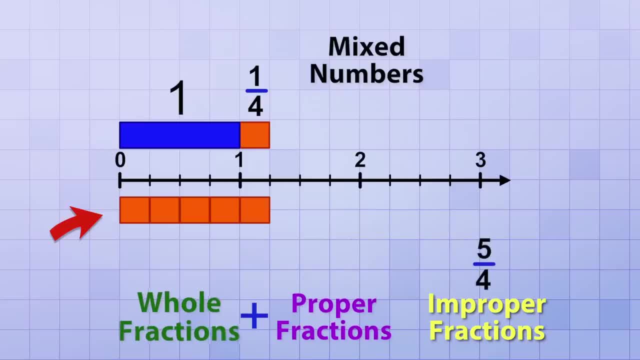 But notice how we got it… we added a proper fraction to a whole fraction. When we just had 4 fourths, we had a whole fraction. But when we added one more fourth it became the improper fraction: 5 over 4.. 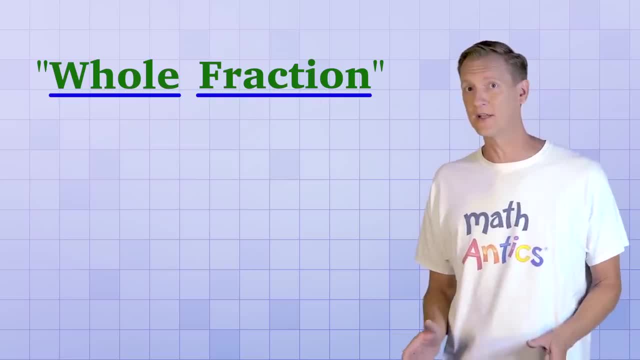 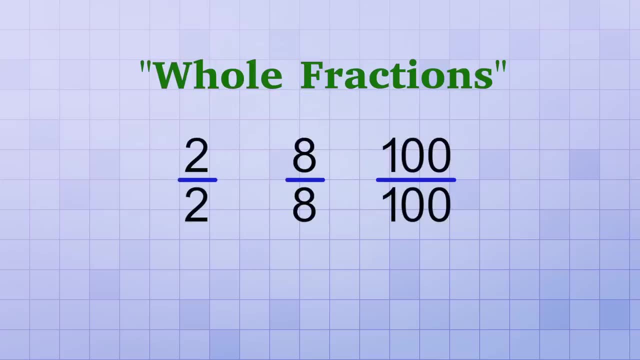 I say whole fraction, I'm talking about any fraction that is equal to 1 whole fraction, Any fraction that has the exact same number on the top and on the bottom: 2 over 2, 8 over 8, 100 over 100… those are all what I call whole fractions. 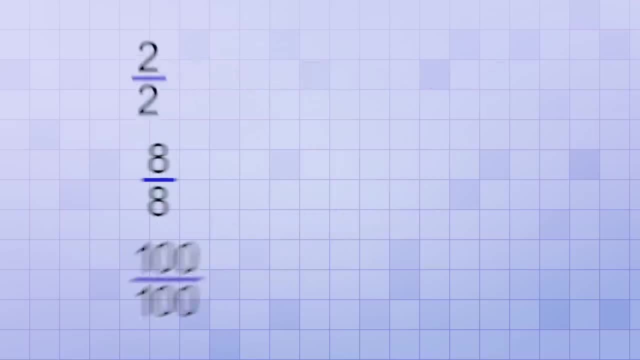 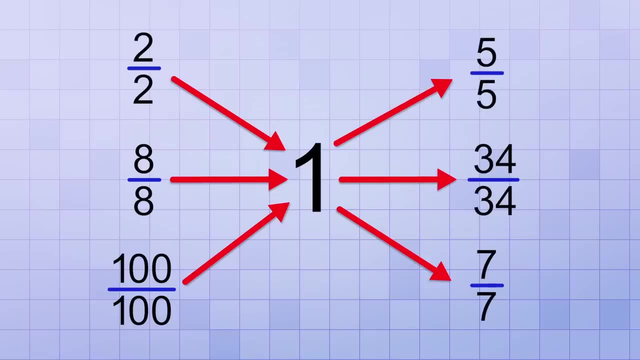 Since all whole fractions equal 1,, you can replace any whole fraction with 1, and you can replace 1 with any whole fraction, And you can see how that works. on our number line, The 4 fourths all combine to cover the same distance as 1.. 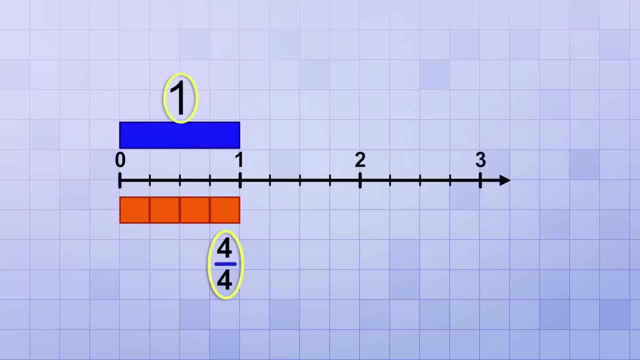 The fraction 4 over 4 is equivalent to 1. And vice versa. But now what if we get a little crazy and add one more fourth? Now we have 5 fourths and we've gone past 1 on the number line. 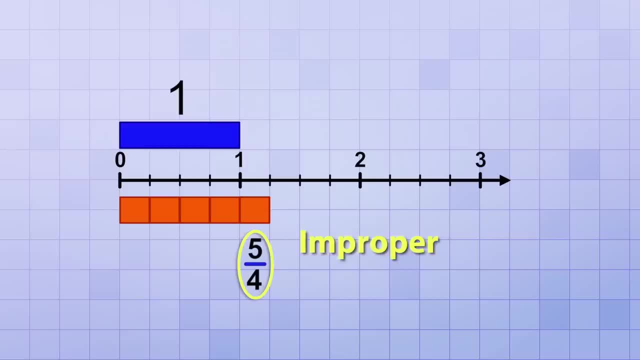 5 fourths or 5 over 4, is what we call an improper fraction, Because the numerator, the top number, is greater than the denominator, the bottom number. That means its value is greater than 1.. In this particular case, how much greater than 1 is it? 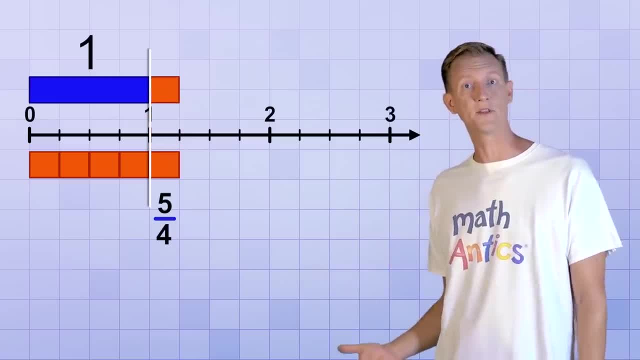 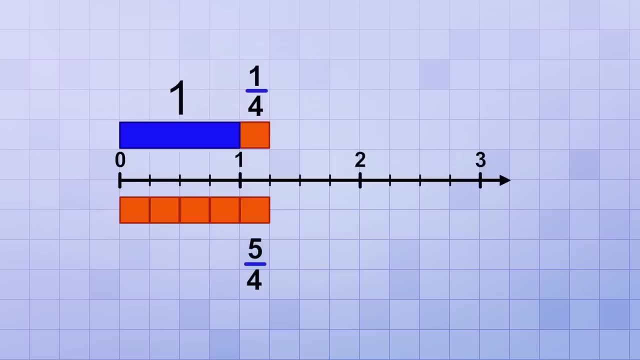 1 by the fractional amount 1- fourth. So 5 fourths turns out to be equivalent to 1 and 1 fourth. Have a good look at this diagram for a minute, because it shows us something really important about how proper fractions, improper fractions, whole fractions and mixed numbers all relate. 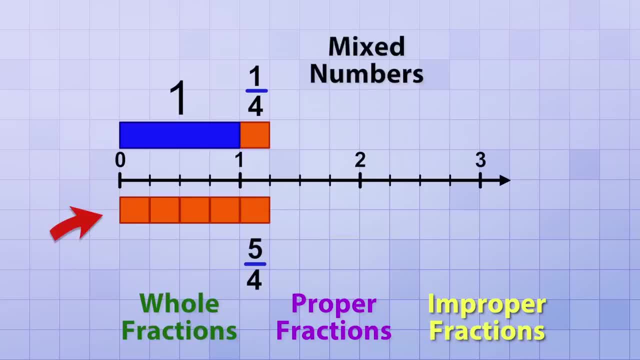 to each other. First, on this side of the number line, we have 5 fourths, which we know is an improper fraction. But notice how we got it… we added a proper fraction to a whole fraction. When we just add 4 fourths, we add a whole fraction. But when we added one more fourth, it became: 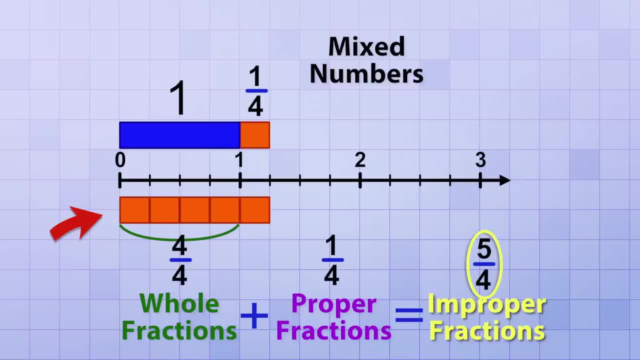 the improper fraction 5 over 4.. So one way to think of an improper fraction is that it's a combination of one or more whole fractions and a proper fraction. That's helpful because we know that all whole fractions can be simplified to the whole. 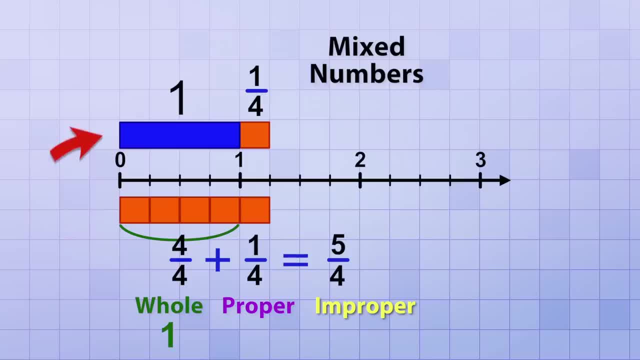 number 1.. And if we did that, we'd get what's shown on the other side of the number line. We'd get the combination of the whole number 1 and the proper fraction 1- fourth. In other words, we'd get a mixed number. 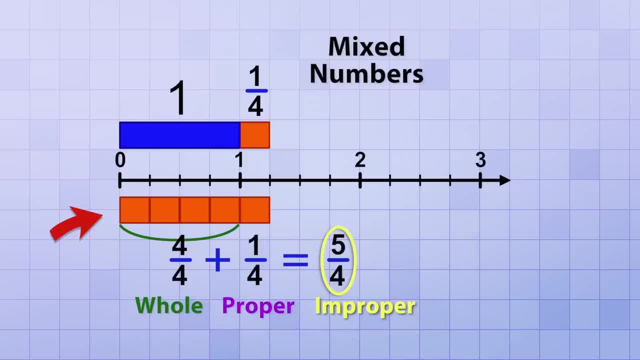 So one way to think of an improper fraction is that it's a combination of one or more whole fractions and a proper fraction. That's helpful, because we know that all whole fractions can be simplified to the whole number 1.. And if we did that, we'd get what's shown on the other side of the number line. 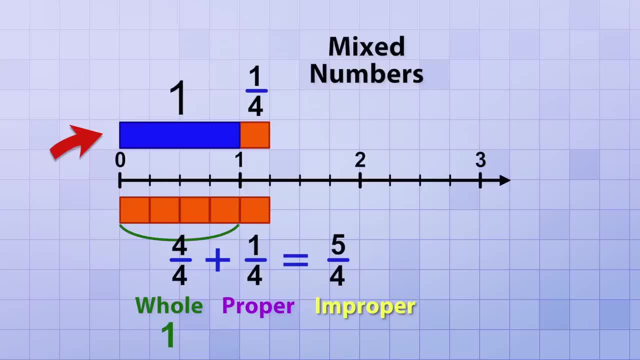 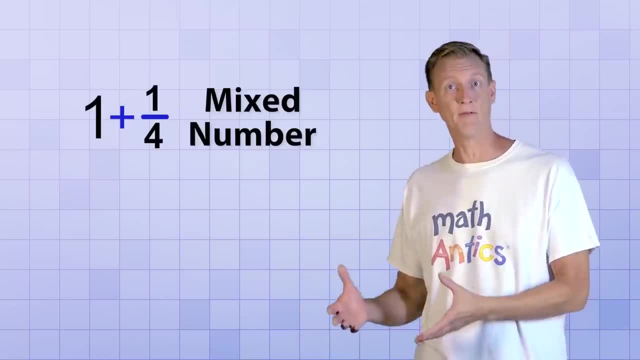 We'd get the combination of the whole number, 1 and the proper fraction, 1- fourth. In other words, we'd get a mixed number. That's all. a mixed number is It's the sum of a whole number and a proper fraction. 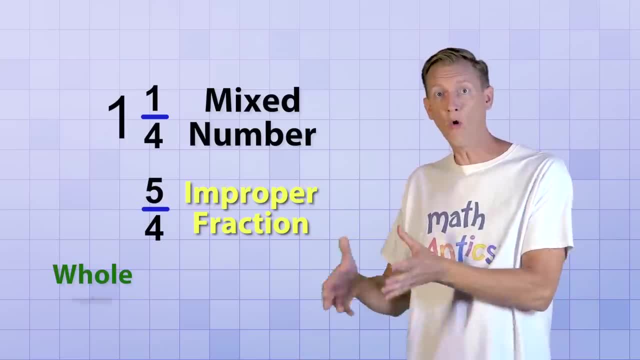 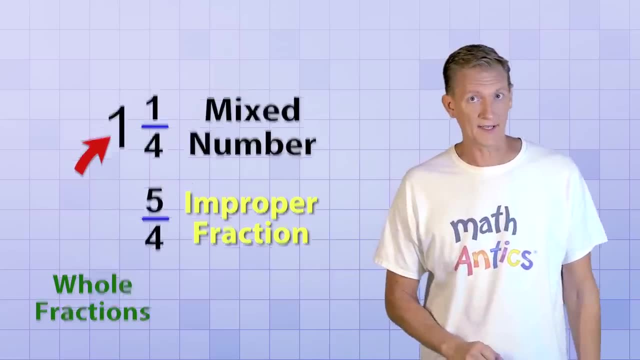 It's an alternate way to write an improper fraction, where all the whole fractions that are inside the improper fraction have been simplified out into a whole number. To help that sink in, let's look at another improper fraction: 8 over 3, or 8 thirds. 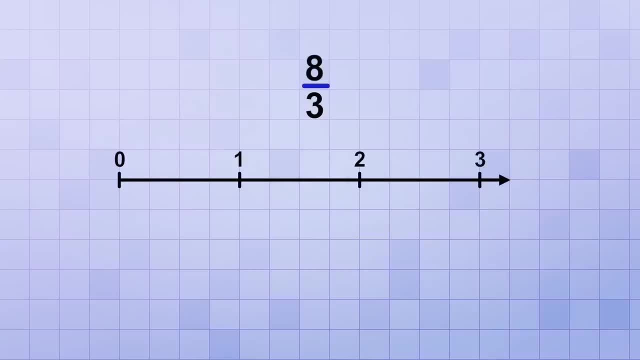 We'll use the same number line that goes from 0 to 3, but this time let's subdivide each whole number into 3 parts to make counting thirds easier. So this would be 1 third, this is 2 thirds and this is 3 thirds. 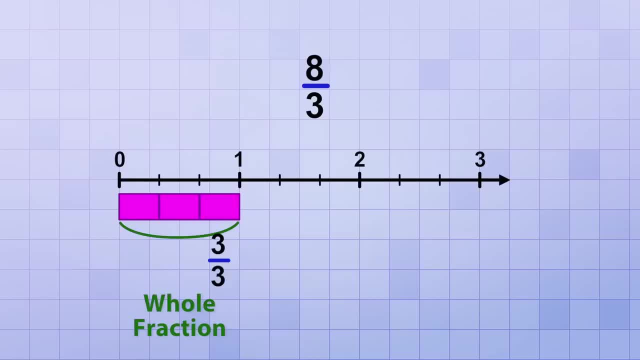 Oh, there's a whole fraction already. Let's make note of that while we continue adding thirds. Next we have 4 thirds, 5 thirds, 6 thirds… Oh, we just formed another group of 3 thirds. That would equal a whole fraction also. 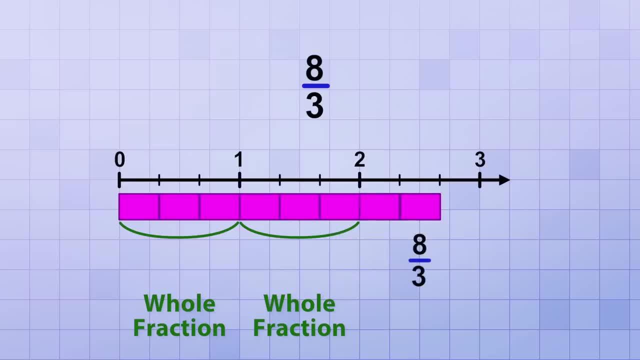 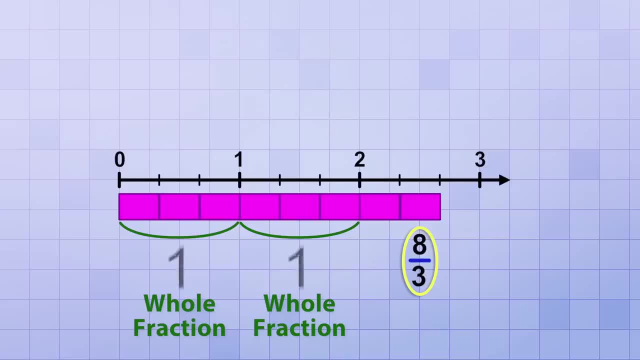 8 thirds actually contain 2 whole fractions. Each of those whole fractions simplifies to 1.. So that means our mixed number form would have 1 plus 1, or 2, as the whole number part, And then the fraction that's left over after simplifying all the whole fractions is 2 thirds. 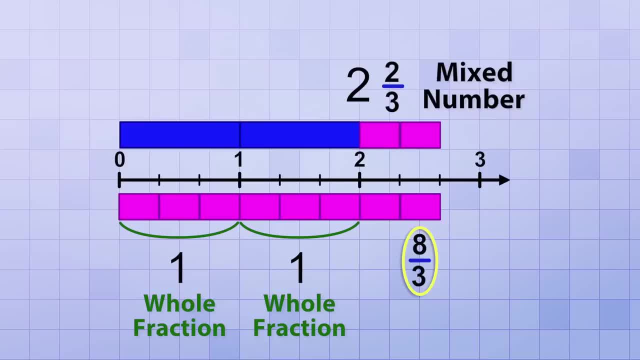 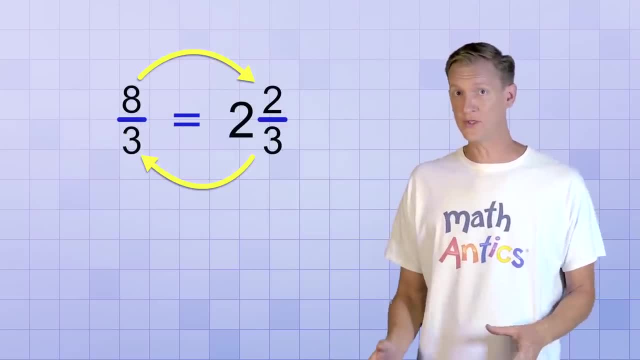 So the improper fraction, 8 thirds, is equivalent to the mixed number 2 and 2 thirds. Pretty cool, huh? And to show you that you can go back and forth between these two forms, check this out In the mixed number 2 and 2 thirds. 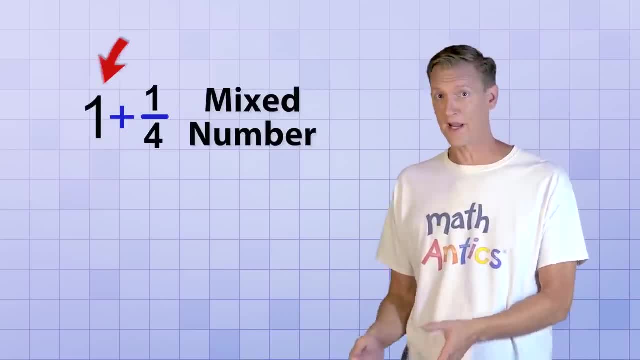 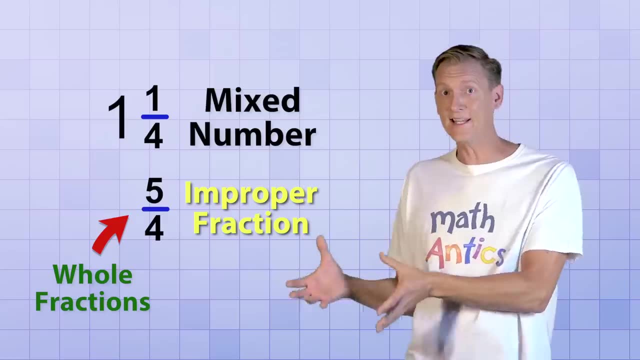 That's all. a mixed number is: It's the sum of a whole number and a proper fraction. It's an alternate way to write an improper fraction, where all the whole fractions that are inside the improper fraction have been simplified out into a whole number. 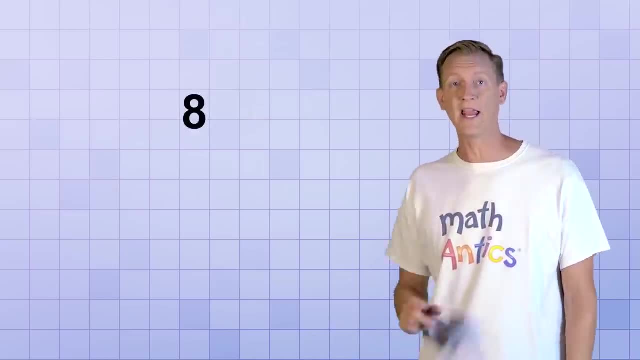 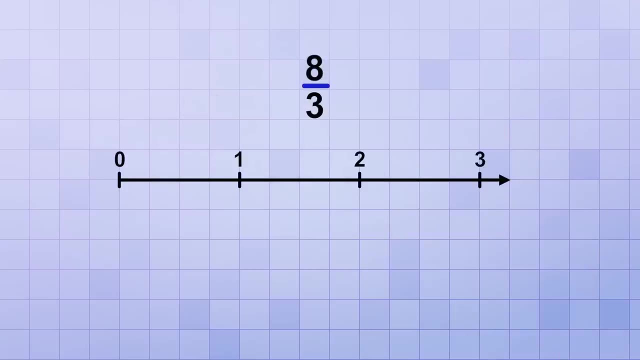 To help that sink in, let's look at another improper fraction: 8 over 3, or 8 thirds. We'll use the same number line that goes from 0 to 3, but this time let's subdivide each whole number into a whole number. 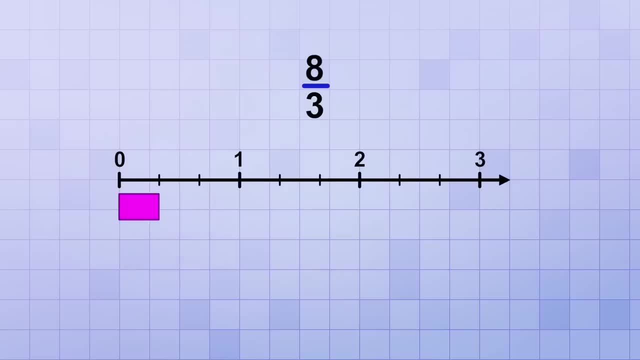 We'll divide the whole number into 3 parts to make counting thirds easier. So this would be 1 third, this is 2 thirds and this is 3 thirds. Oh, there's a whole fraction already. Let's make note of that while we continue adding thirds. 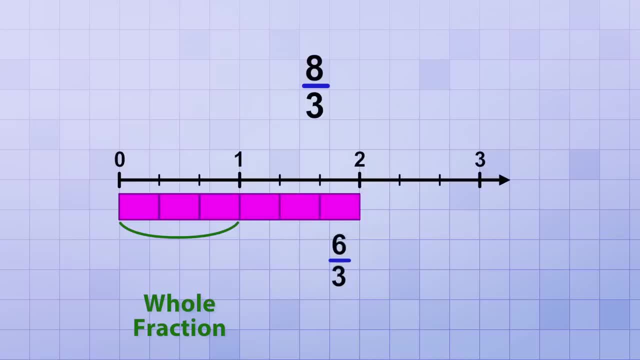 Next we have 4 thirds, 5 thirds, 6 thirds… oh, we just formed another group of 3 thirds That would equal a whole fraction. also, Let's note that, and continue… 7 thirds and 8 thirds. As we noted, 8 thirds actually contain 2 whole fractions. 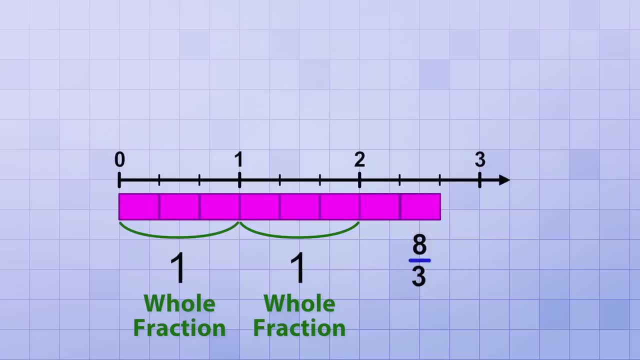 Each of those whole fractions simplifies to 1,, so that means our mixed number form would have 1 plus 1, or 2, as the whole number part, And then the fraction that's left over after simplifying all the whole fractions is 2 thirds. 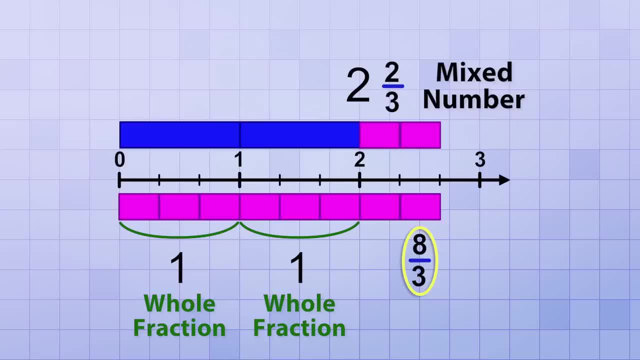 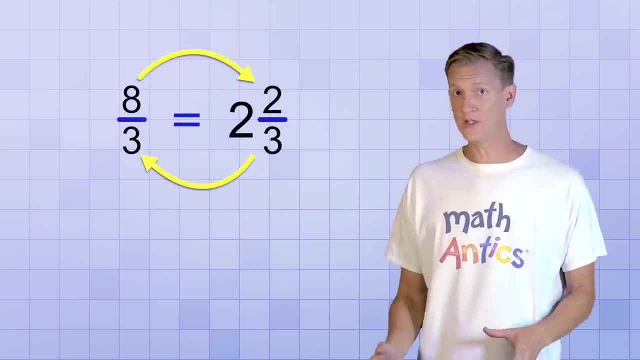 so the improper fraction, 8 thirds, is equivalent to the mixed number 2 and 2 thirds. Pretty cool, huh. And to show you that you can go back and forth between these two forms, check this out: In the mixed number 2 and 2 thirds, the whole number is 1.. 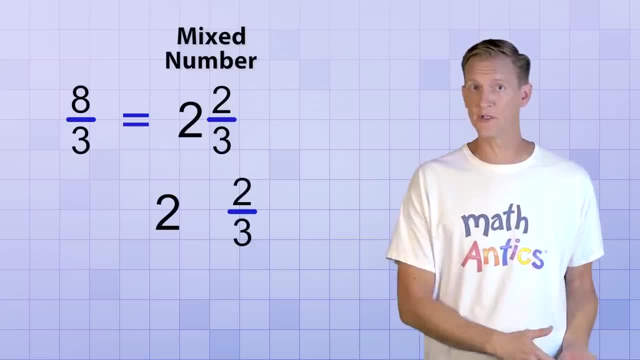 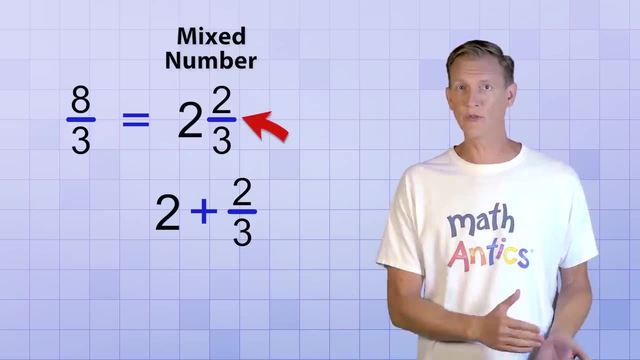 the whole number 2, and the fraction 2 thirds are being added together. That's really important to know, even though the plus sign isn't usually shown. So 2 and 2 thirds is really 2 plus 2 thirds. 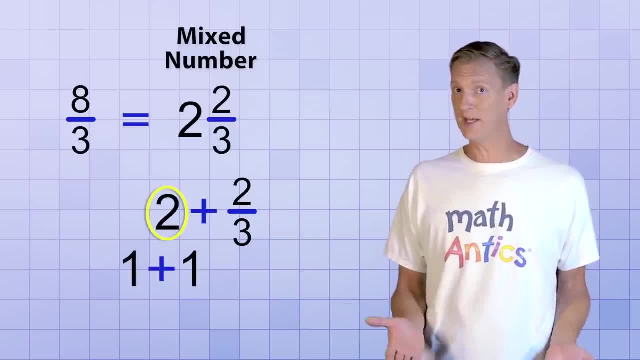 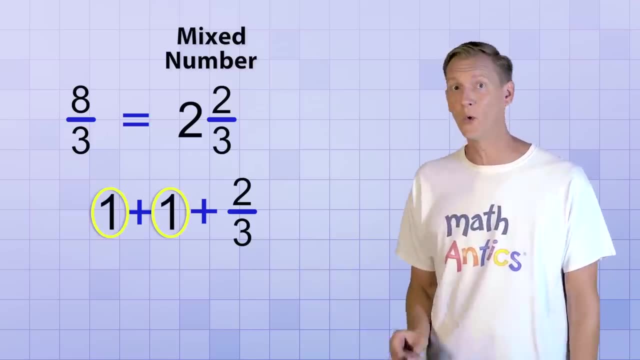 And if we wanted to, we could expand the 2 into 1 plus 1, right, That gives us 1 plus 1 plus 2 thirds. And then we could replace each of those 1's with the whole fraction 3 over 3, since 3 over 3 equals 1.. 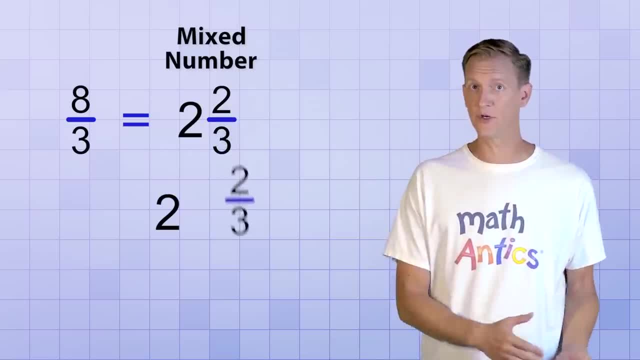 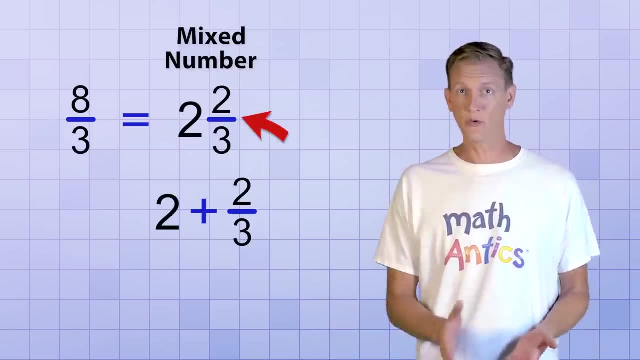 In the mixed number 2 and 2 thirds, the whole number 2, and the fraction 2 thirds are being added together. That's really important to know, even though the plus sign isn't usually shown. So 2 and 2 thirds is really 2 plus 2 thirds. 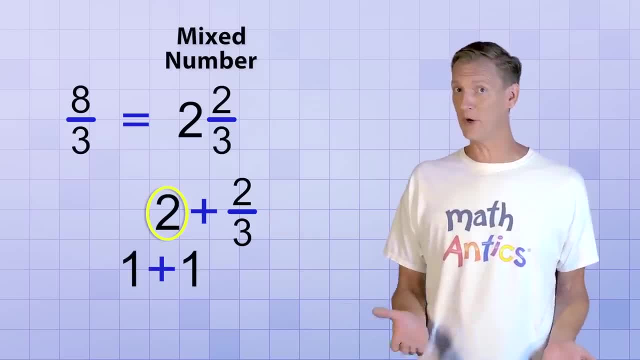 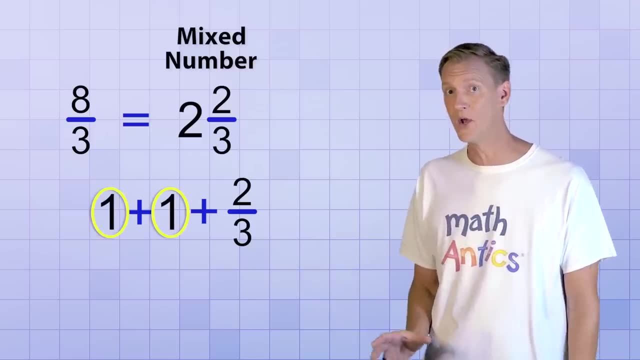 And if we wanted to, we could expand the 2 into 1 plus 1, right, That gives us 1 plus 1 plus 2 thirds. And then we could replace each of those 1's with the whole fraction 3 over 3, since 3 over 3 equals 1.. 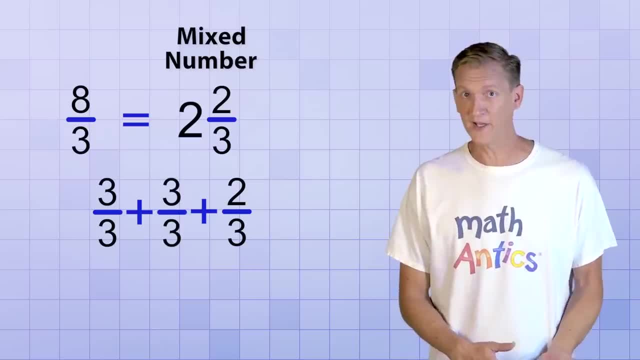 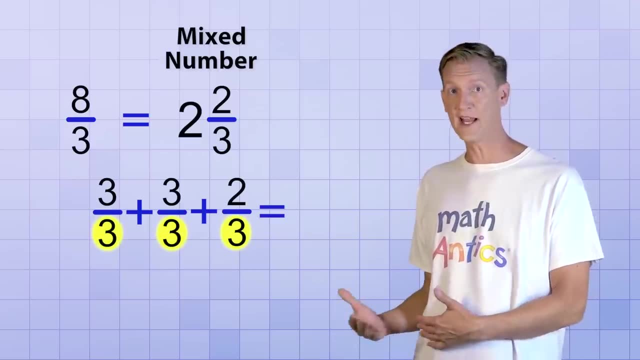 That gives us 3 over 3 plus 3 over 3 plus 2 over 3.. Since these fractions all have the same denominator, we can add them easily. The denominator of the answer will stay the same- 3,- and the numerator will be the sum of the other numerators. 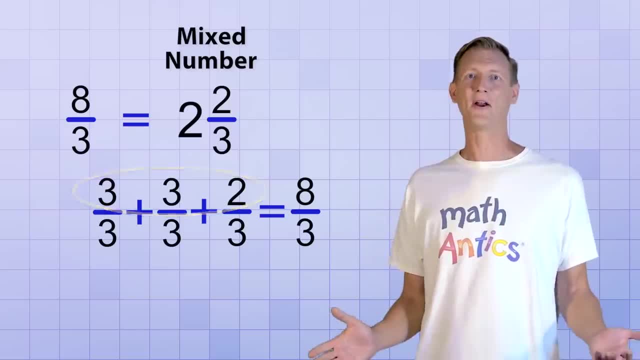 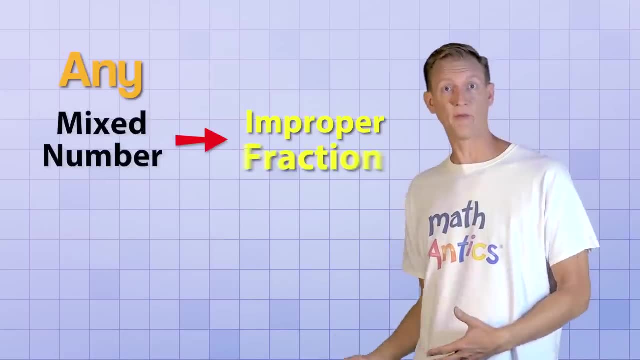 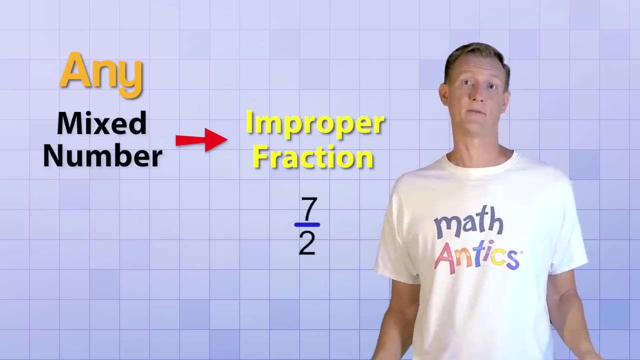 3 plus 3 plus 2 equals 8.. And there we are Back to our original improper fraction: 8 over 3.. You can convert any mixed number into an improper fraction using that procedure. You can change the whole number part into a sum of whole fractions and then add everything up. 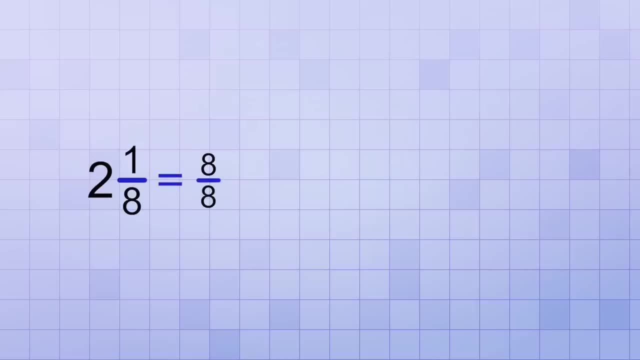 For example, 2 and 1 eighth could be changed into 8 over 8 plus 8 over 8 plus 1 over 8, which all add up to 17 over 8.. And 3 and 4 fifths could be changed to 5 over 5 plus 5 over 5 plus 5 over 5 plus 4 over 5,. 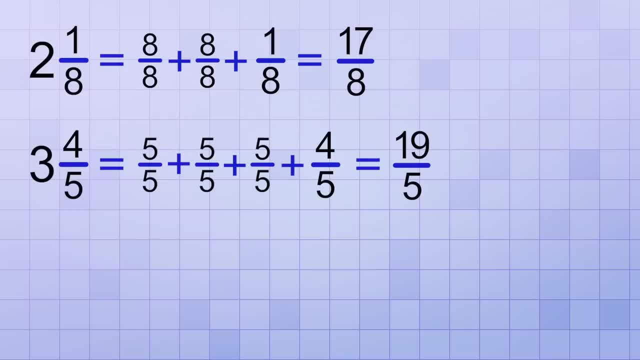 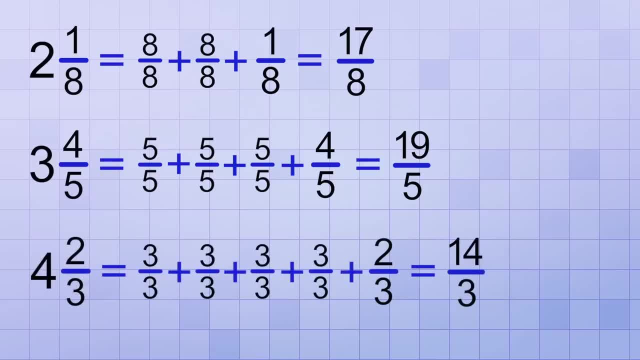 which all adds up to 14 over 3.. Notice that we always chose whole fractions with the same denominator of the fraction, part of the mixed number, so that they're all like fractions that can be added easily And some of you might see the shortcut here. 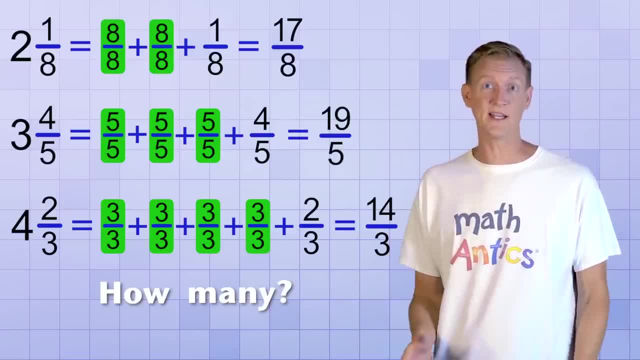 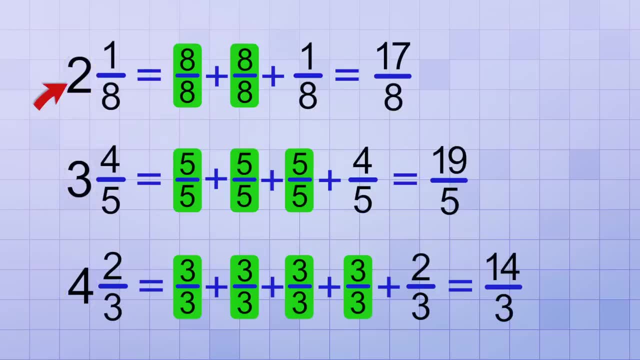 In each case. did you notice how many of the whole fractions we needed to add together? Yep, it's the same as the whole number, part of the mixed number. If it's 2,, then we need to add 2 whole fractions. 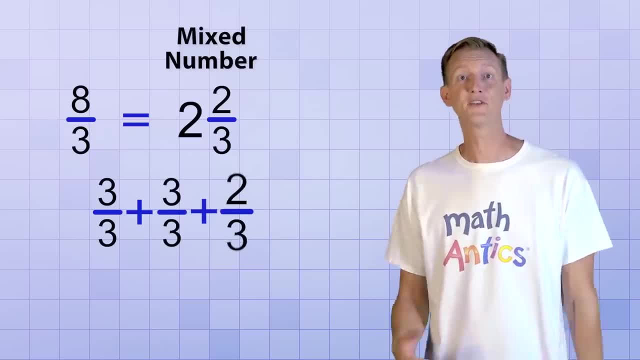 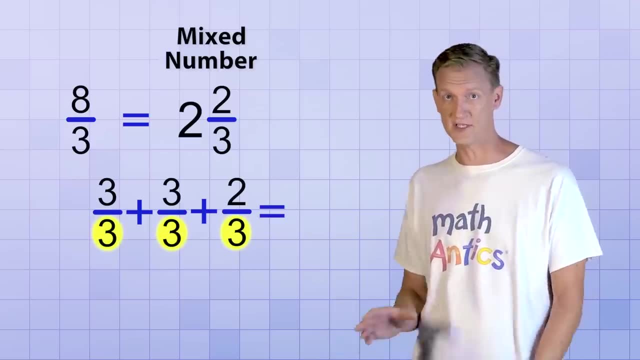 That gives us 3 over 3 plus 3 over 3 plus 2 over 3.. Since these fractions all have the same denominator, we can add them easily. The denominator of the answer will stay the same- 3,- and the numerator will be the sum of the other numerators. 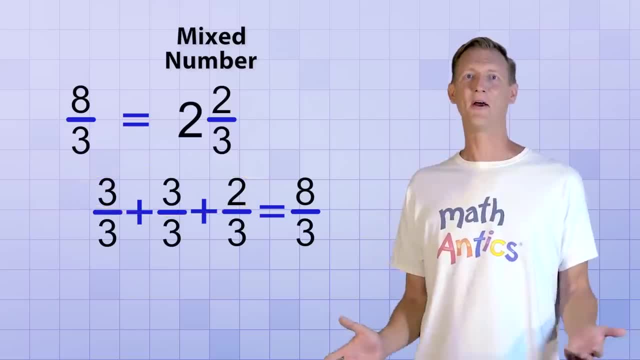 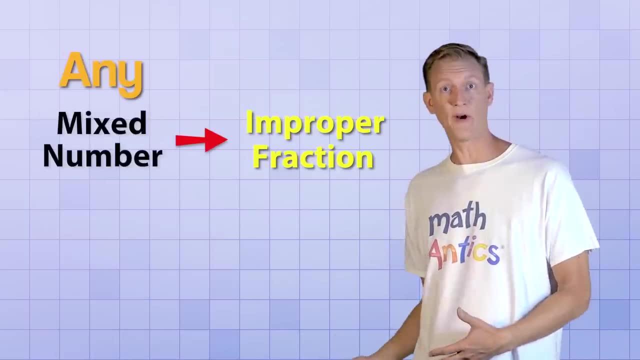 3 plus 3 plus 2 equals 8.. And there we are back to our original improper fraction: 8 over 3.. You can convert any mixed number into an improper fraction using that procedure. You can change the whole number part. 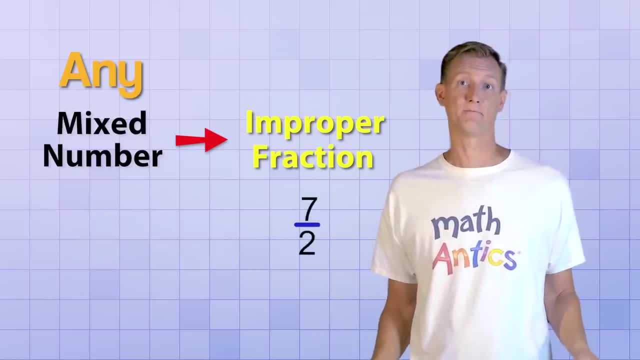 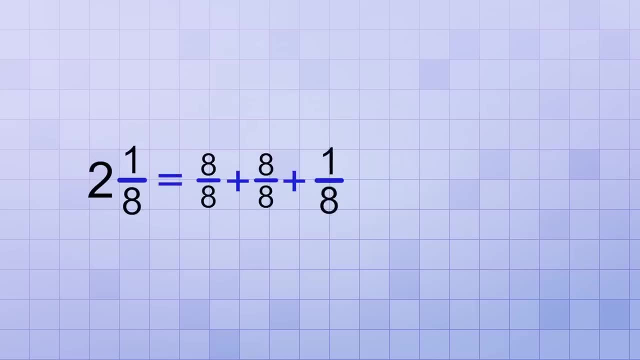 into a sum of whole fractions and then add everything up. For example, 2 and 1 eighth could be changed into 8 over 8 plus 8 over 8 plus 1 over 8, which all add up to 17 over 8.. 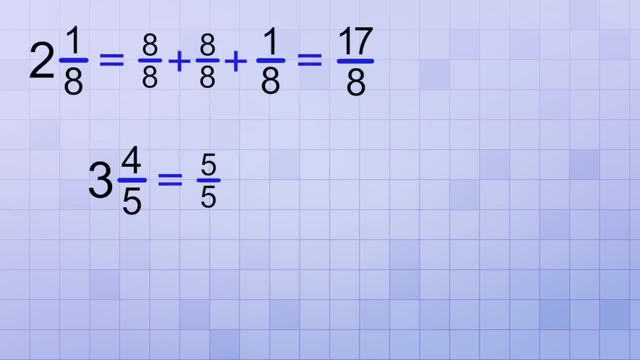 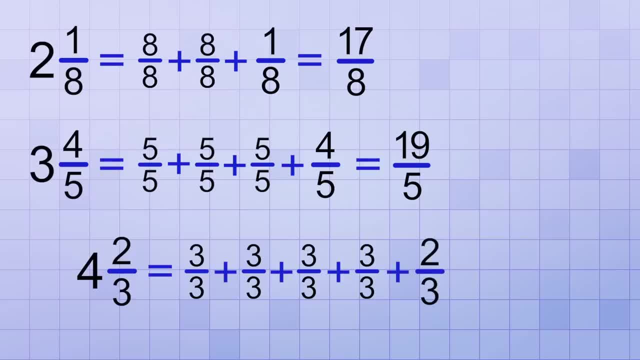 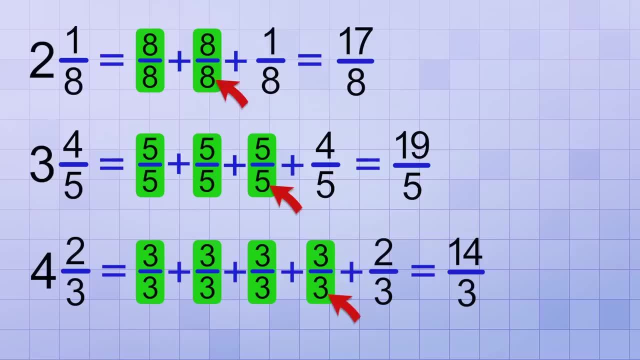 plus 3 over 3 plus 3 over 3 plus 2 over 3, which all adds up to 14 over 3.. Notice that we always chose whole fractions with the same denominator of the fraction, part of the mixed number, so that they're all like fractions that can be added easily. 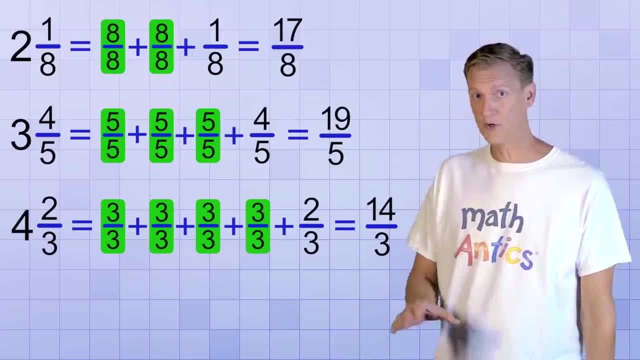 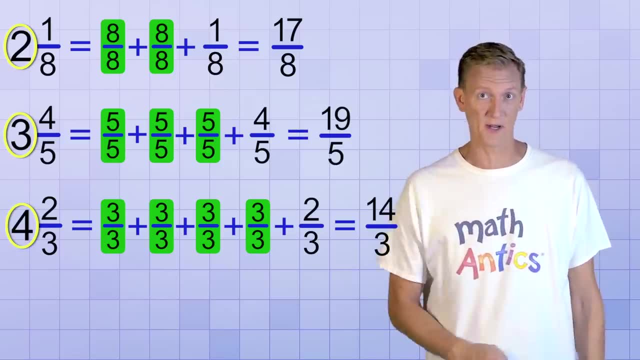 And some of you might see the shortcut here. In each case, did you notice how many of the whole fractions we needed to add together? Yup, it's the same as the whole number, part of the mixed number. If it's 2,, then we need to add up the whole fractions. 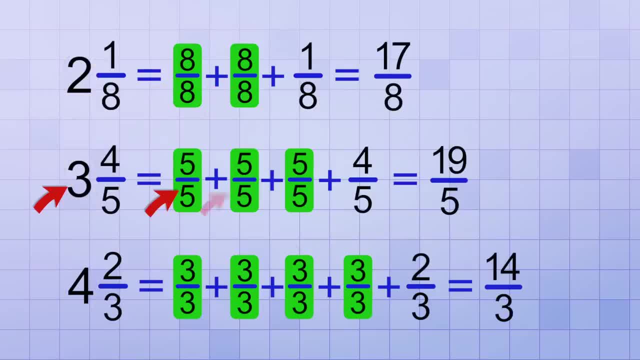 If it's 3,, we need to add 2 whole fractions. If it's 3,, we need to add 3 whole fractions. If it's 4, we need to add 4 whole fractions, And so on. The whole number tells us how many times to repeat the addition. 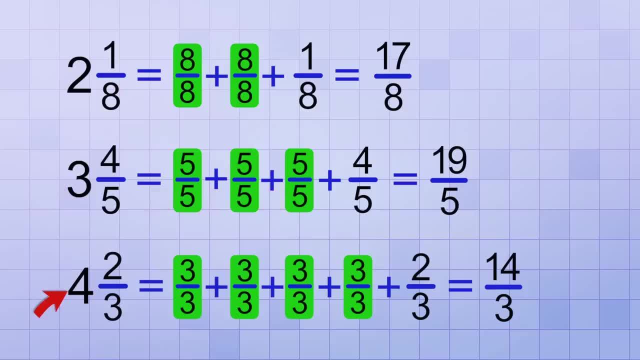 If it's 3,, we need to add 3 whole fractions. If it's 4, we need to add 4 whole fractions, And so on. The whole number tells us how many times to repeat the addition And since multiplication is repeated addition, we can multiply instead of adding. 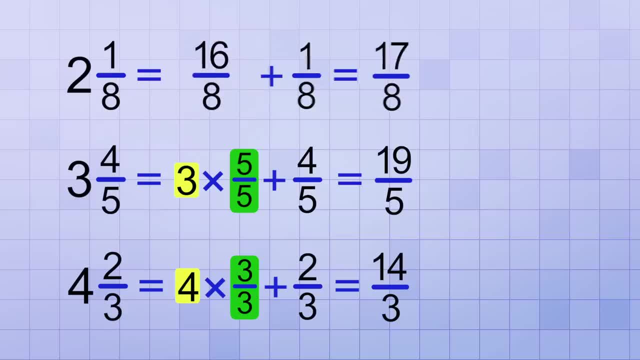 2 times 8 over 8 gives us 16 over 8, and then we add that result to 1 over 8 to get 17 over 8.. 3 times 5 over 5 gives us 15 over 8.. 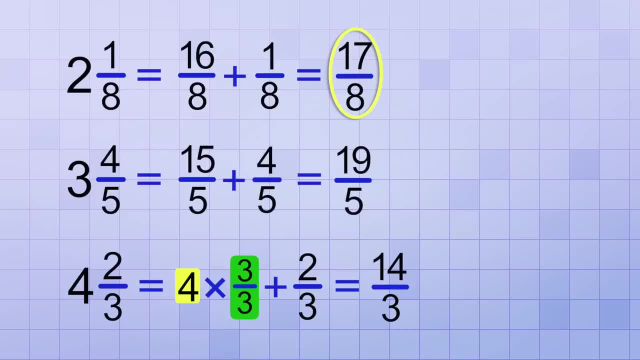 3 times 5 over 5 gives us 15 over 8.. 3 times 5 over 5 gives us 15 over 8, and then we add that result to 4 over 5 to get 19 over 5.. 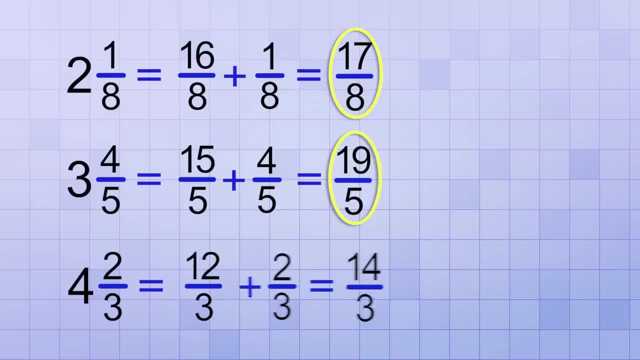 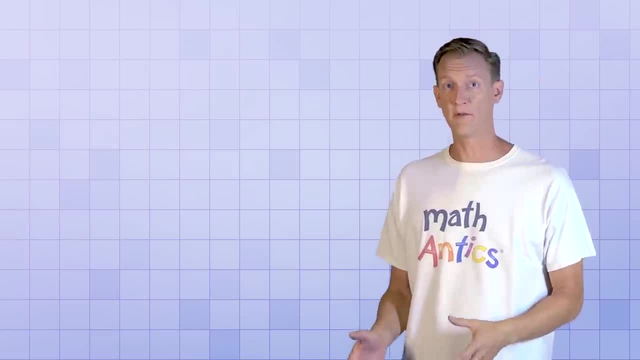 4 times 3 over 3 gives us 12 over 3, and then we add that result to 2 over 3 to get 14 over 3.. That shortcut really helps when the whole number, part of the mixed number, is big. 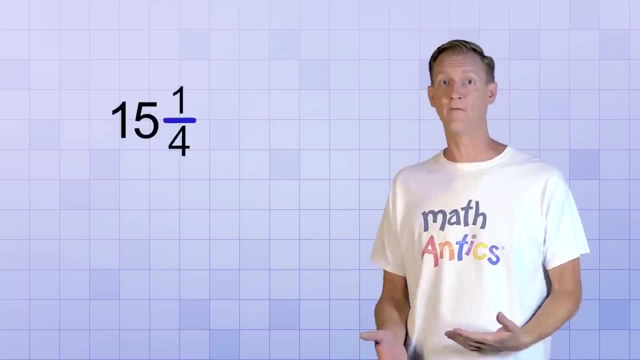 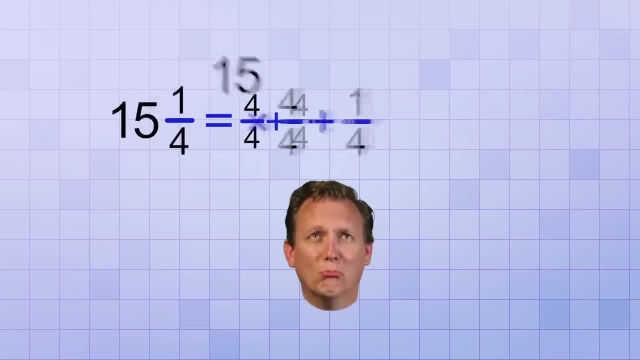 Like what if we needed to convert the mixed number 15 and 1- fourth into an improper fraction? Instead of having to add 15 whole fractions together, we can just multiply 15 by the whole fraction of 15.. We multiply the whole fraction 4 over 4, which gives us 60 over 4.. 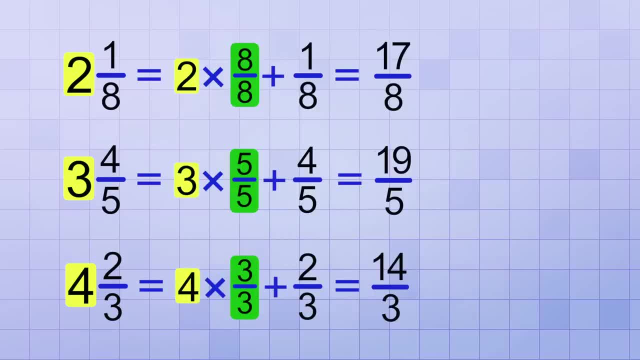 And since multiplication is repeated addition, we can multiply instead of adding. 2 times 8 over 8 gives us 16 over 8, and then we add that result to 1 over 8 to get 17 over 8.. 3 times 5 over 5 gives us 15 over 5,. 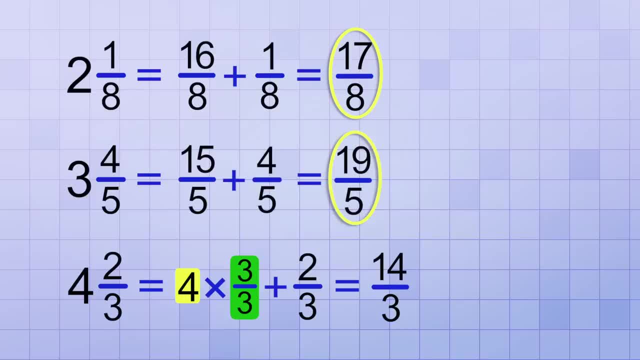 and then we add that result to 1 over 8 to get 17 over 8.. And then we add that result to 4 over 5 to get 19 over 5.. 4 times 3 over 3 gives us 12 over 3, and then we add that result to 2 over 3 to get 14 over 3.. 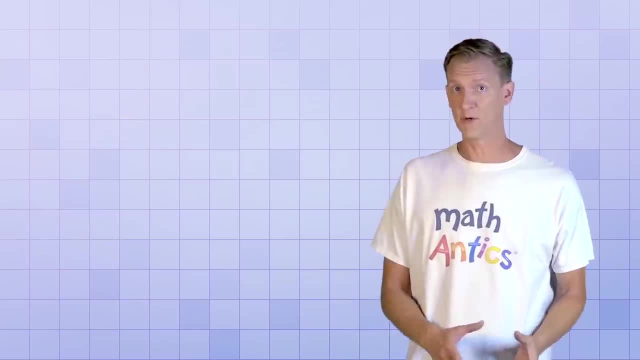 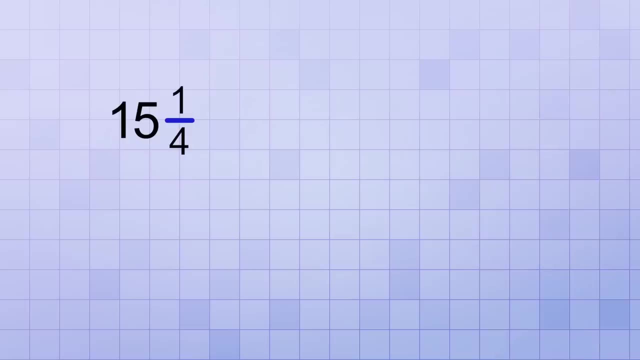 That shortcut really helps when the whole number, part of the mixed number, is big. Like what if we needed to convert the mixed number 15 and 1 fourth into an improper fraction? Instead of having to add 15 whole fractions together, we can just multiply 15 by the whole fraction, 4 over 4,. 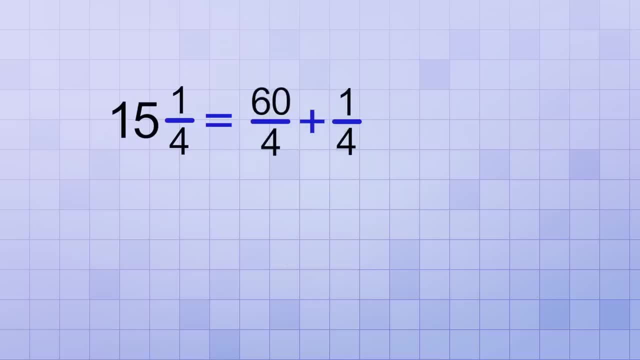 which gives us 60 over 4.. Then we add that result to the fraction 1 over 4 to get 61 over 4.. That's the improper fraction form of 15 and 1 fourth. Alright then, but what if we need to go the other way? 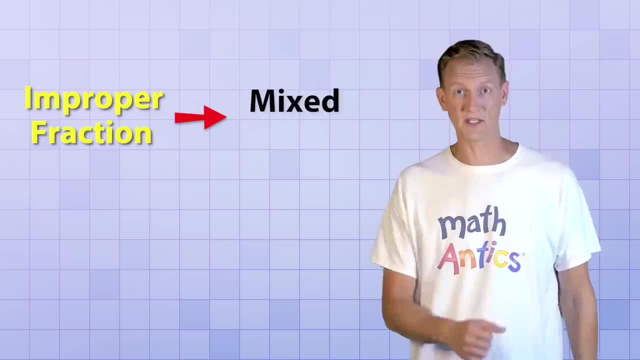 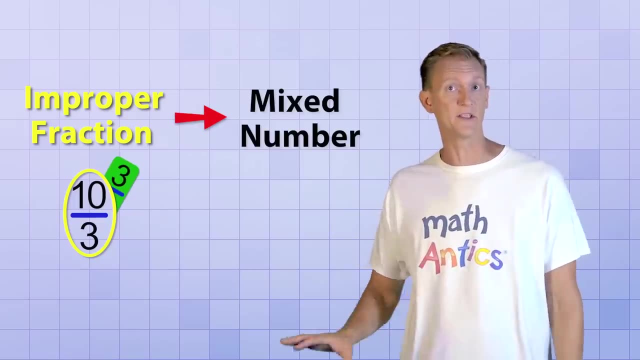 What if we start with an improper fraction and need to convert it into a mixed number? Well, whenever we have an improper fraction, we know there's at least one whole fraction hiding in there that we could simplify out. The question is, how many? 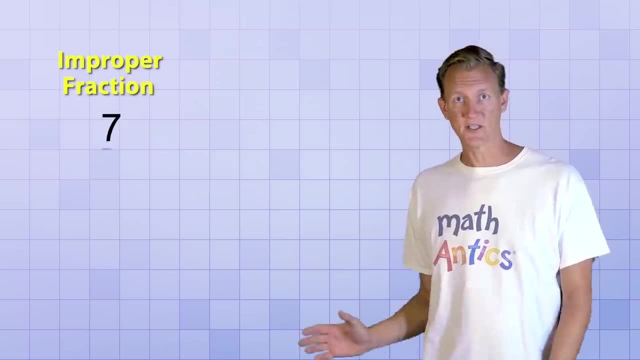 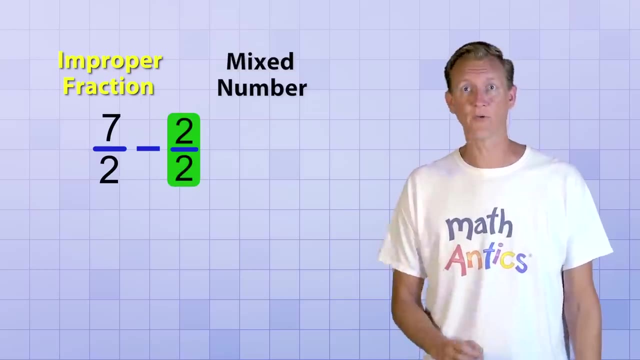 To see what I mean, let's try converting the whole number into a mixed number. Let's start by converting the improper fraction 7 over 2 into a mixed number, using a little trial and error. First, let's try subtracting out just one whole fraction. 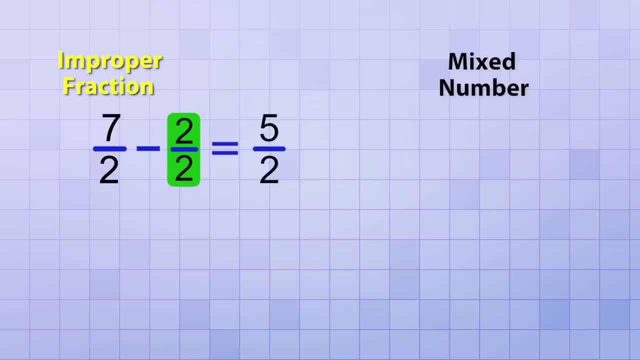 7 over 2 minus 2 over 2 equals 5 over 2.. That means we can write 7 over 2 as the mixed number 1 and 5 over 2, since we subtracted out one whole fraction and had 5 over 2 left over. 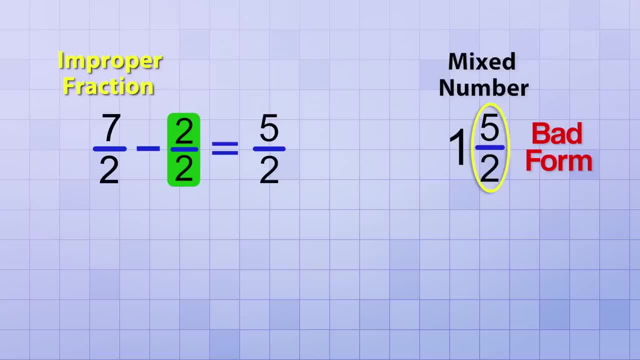 And even though that's true, it's bad form because 5 over 2 is still an improper fraction, which means that there's at least one more whole fraction left over. There's more whole fraction hiding in there that we could have subtracted out. 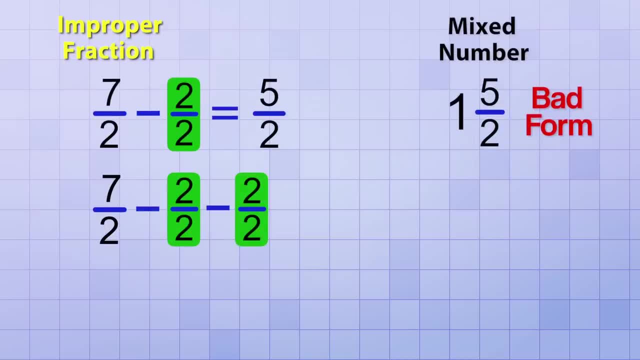 So let's try again, but this time let's subtract out two whole fractions: 7 over 2 minus 2 over 2 minus 2 over 2 equals 3 over 2.. That means we could write 7 over 2 as the mixed number 2 and 3 over 2. 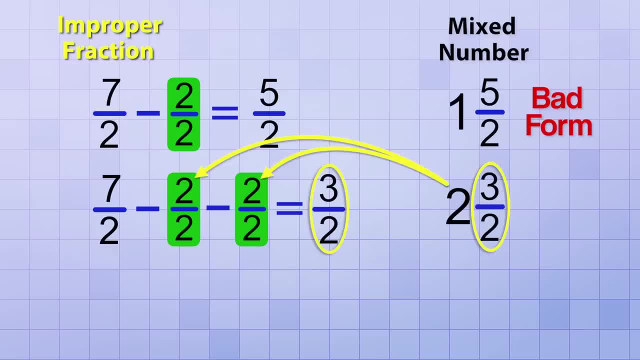 since we subtracted out two whole fractions and had 3 over 2 left over. But that's still bad form because the fraction part is still improper. We could have subtracted out another whole fraction, Subtracting 3 whole fractions this time. 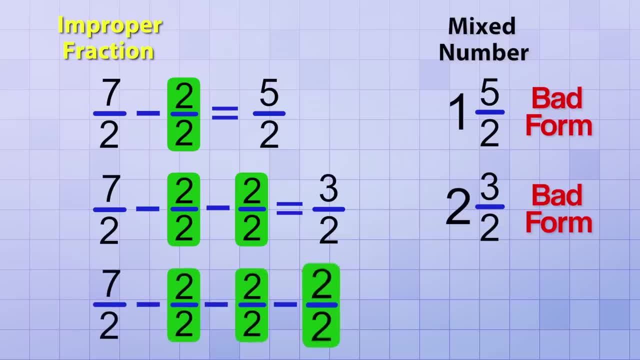 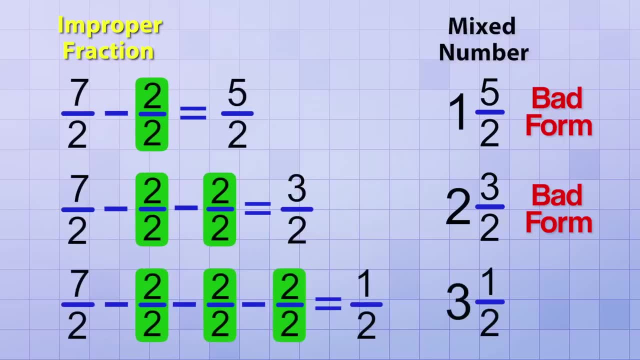 7 over 2 minus 2 over 2 minus 2 over 2 minus 2 over 2 equals 1 half. That means we could write 7 over 2 as the mixed number 3 and 1 half, since we subtracted out 3 whole fractions and had 1 half left over. 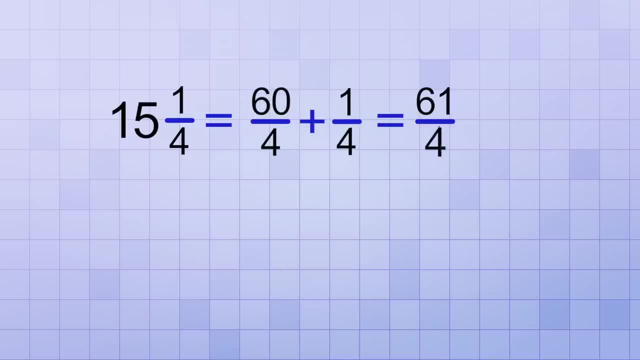 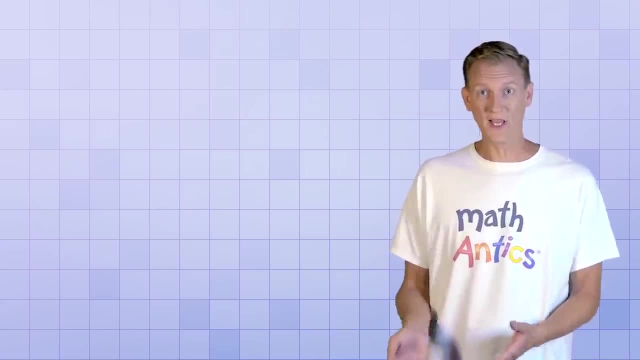 Then we add that result to the fraction 1 over 4 to get 61 over 4.. That's the improper fraction form of 15 and 1 fourth. Alright, then, but what if we need to go the other way? What if we start with an improper fraction and need to convert it into a mixed number? 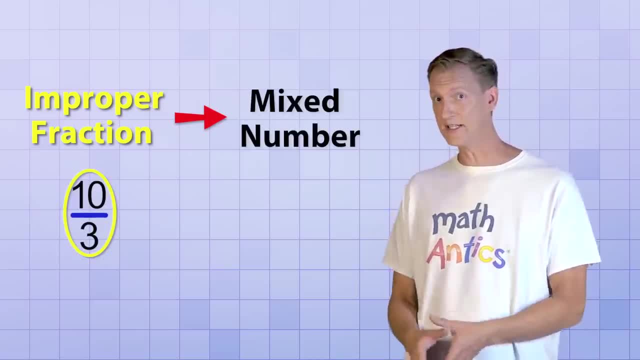 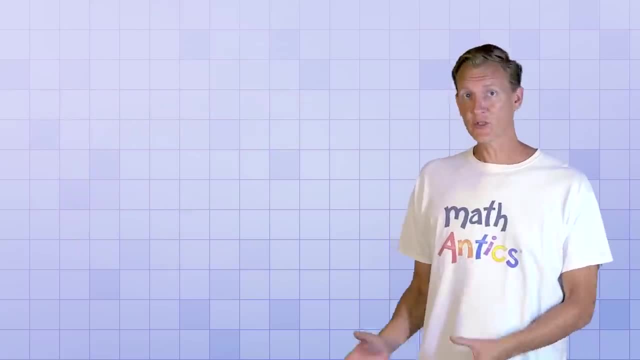 Well, whenever we have an improper fraction, we know there's at least one whole fraction hiding in there that we could simplify out. The question is, how many? To see what I mean, let's try converting the improper fraction 7 over 2 into a mixed number using a little trial and error. 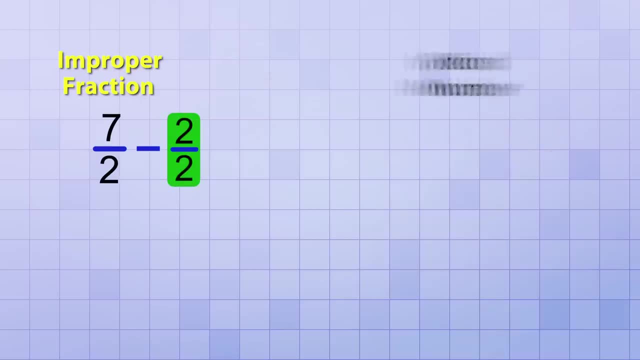 First let's try subtracting out just one whole fraction: 7 over 2 minus 2 over 2 equals 5 over 2.. That means we can write 7 over 2 as the mixed number 1 and 5 over 2. 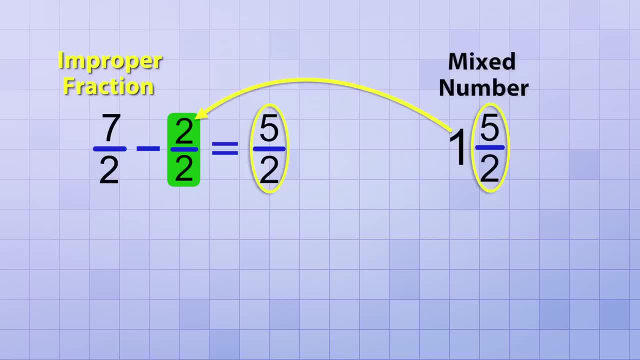 since we subtracted out one whole fraction and had 5 over 2 left over. And even though that's true, it's bad form because 5 over 2 is still an improper fraction, which means that there's at least one more whole fraction hiding in there that we could have subtracted out. 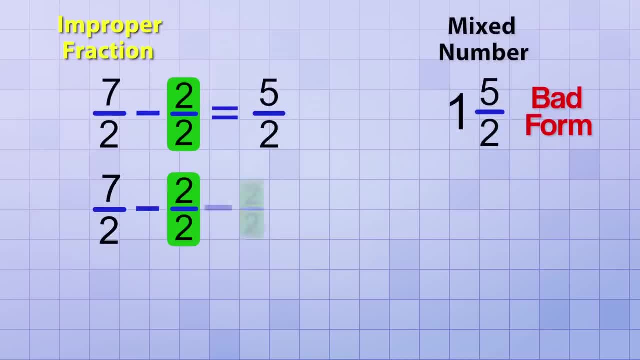 So let's try again, but this time let's subtract out two whole fractions: 7 over 2 minus 2 over 2 minus 2 over 2 equals 3 over 2.. That means we could write 7 over 2 as the mixed number 2 and 3 over 2. 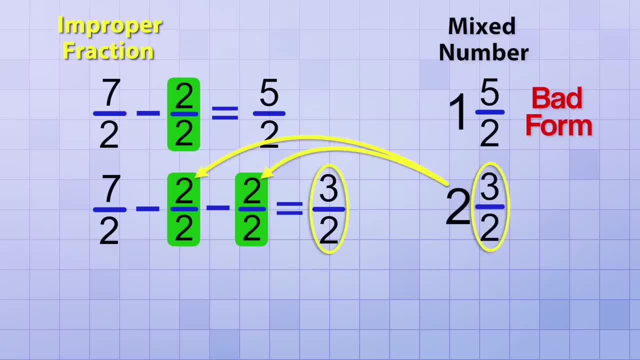 since we subtracted out two whole fractions and had 3 over 2 left over. But that's still bad form because the fraction part is still improper. We could have subtracted out another whole fraction. So let's try again, subtracting three whole fractions this time. 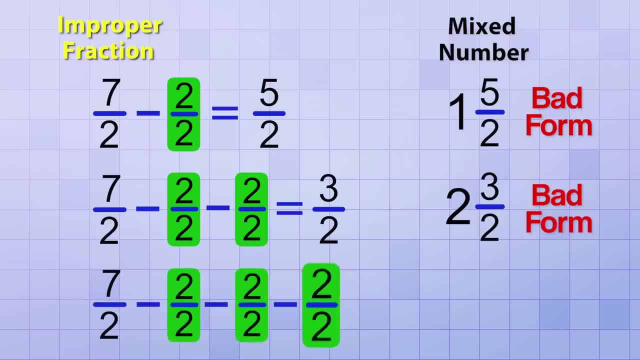 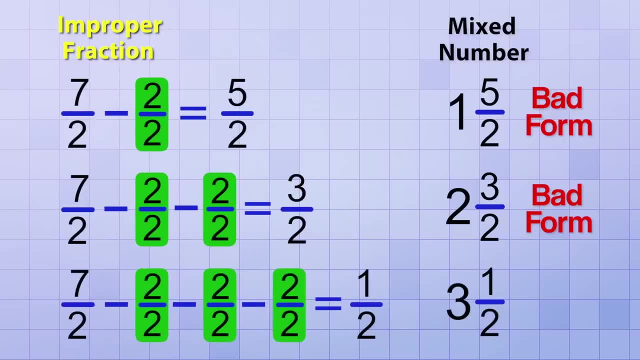 7 over 2 minus 2 over 2 minus 2 over 2 minus 2 over 2 equals 1 half. That means we could write 7 over 2 as the mixed number 3 and 1 half, since we subtracted out three whole fractions and had 1 half left over. 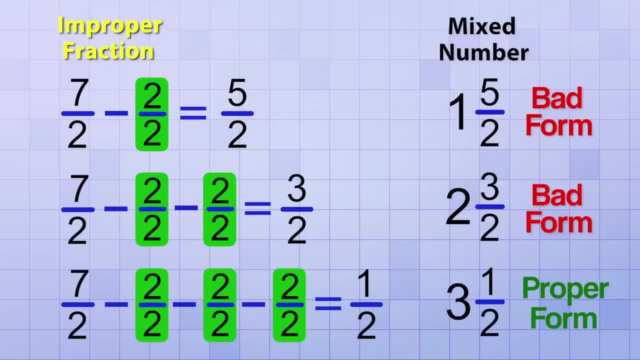 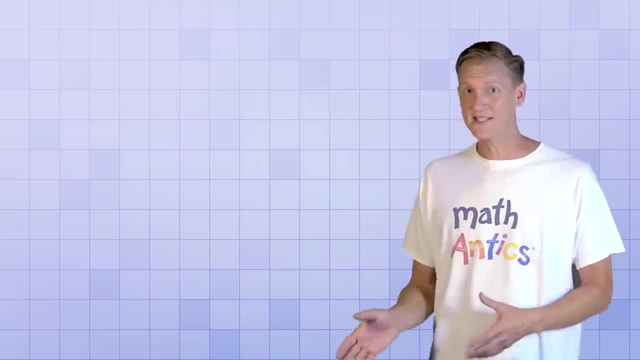 And that's the proper mixed number form of 7 over 2, because it's a whole number and a proper fraction. so there's no more whole fractions that we could simplify out. That process makes sense but it's kind of messy having to subtract out so many whole fractions. 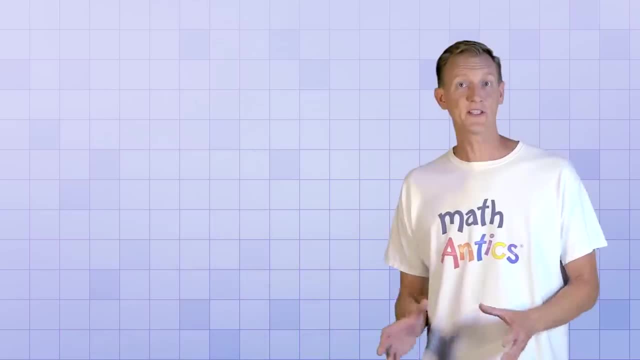 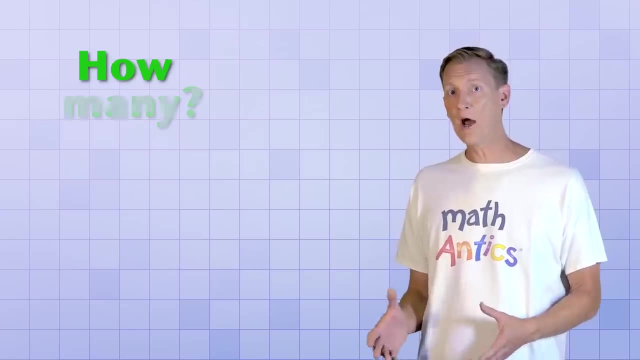 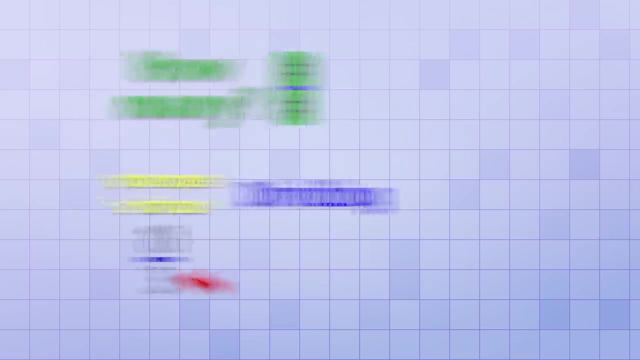 It turns out, there's a shortcut we can take here too. Just like multiplication is repeated addition, division is basically repeated subtraction. That means we can figure out how many whole fractions we can subtract out of an improper fraction by just dividing the top number by the bottom number. 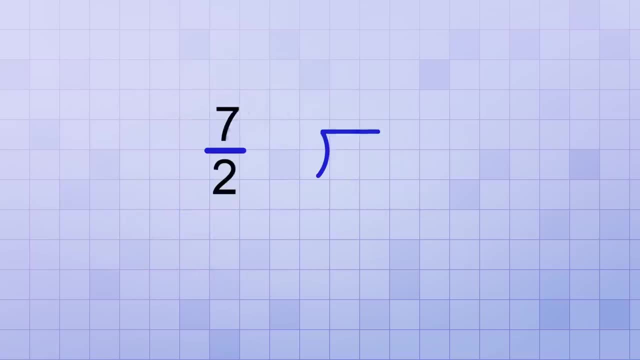 Let's do that with our example 7 over 2.. If we divide 7 by 2, we find out that 2 will divide into 7 three times, leaving a remainder of 1.. That remainder is actually important, as we'll see in a minute. 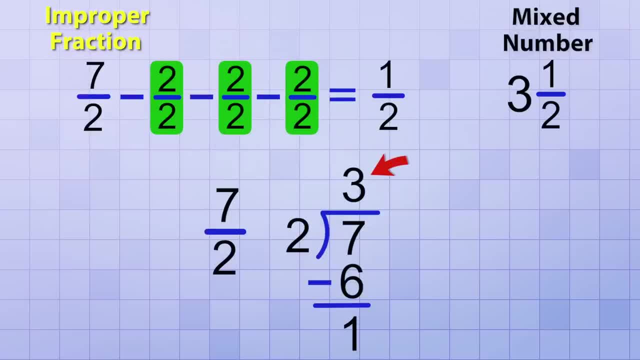 Notice that the answer to our division problem is exactly how many whole fractions we were able to subtract out of the improper fraction 3.. So the answer to the division tells us what the whole number part of the mixed number will be. And here's the really cool part. 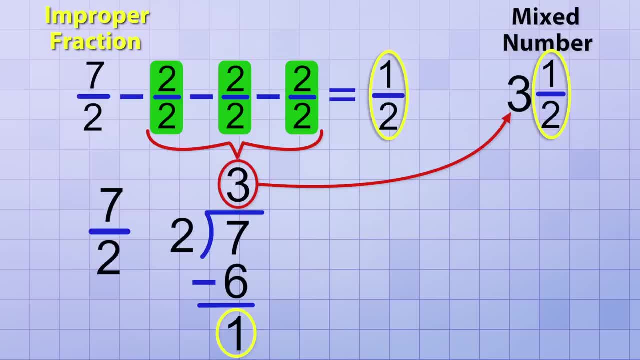 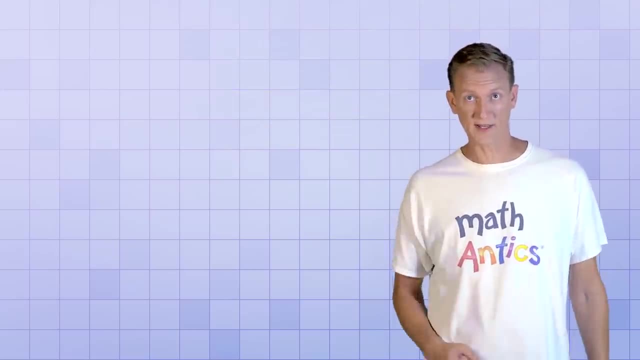 The remainder of the division tells us what the leftover fraction will be. The remainder is the numerator of the leftover fraction. In this case, since the remainder is 1, we'll have 1 over 2 left over in our mixed number. Let's do one more example to make sure you've got that. 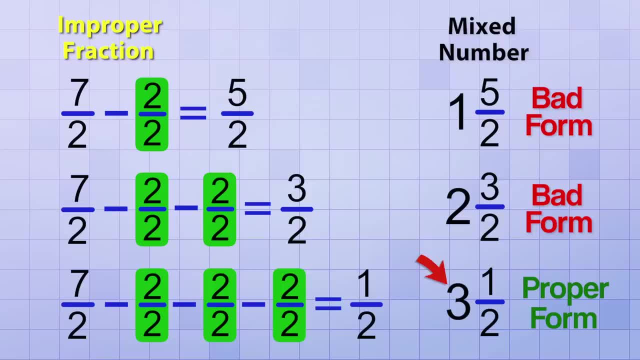 And that's the proper mixed number form of 7 over 2, because it's a whole number and a proper fraction. so there's no more whole fractions that we could simplify out. That process makes sense but it's kind of messy having to subtract out so many whole fractions. 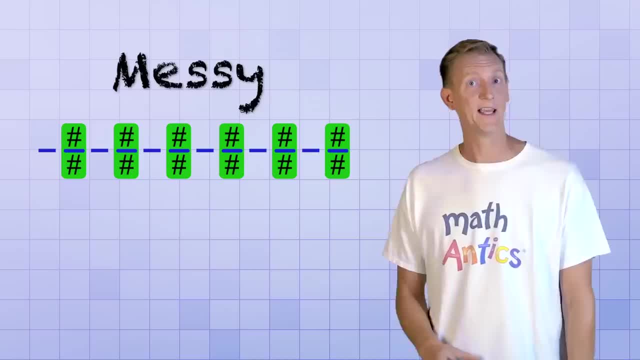 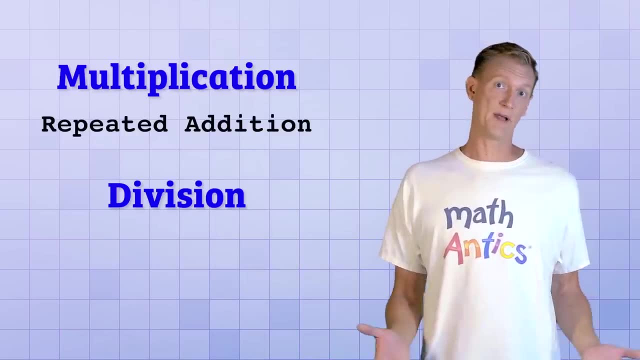 But it's kind of messy having to subtract out so many whole fractions. But it's kind of messy having to subtract out so many whole fractions. It turns out there's a shortcut we can take here too. Just like multiplication is repeated addition, division is basically repeated subtraction. 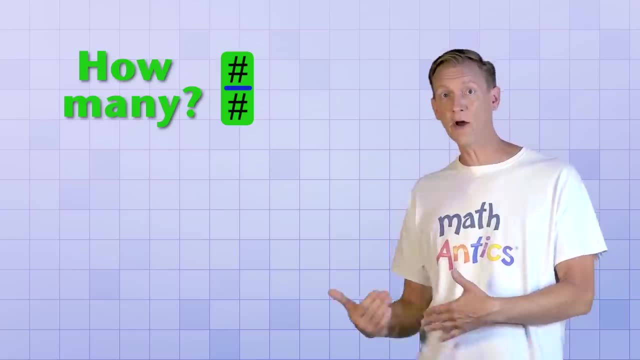 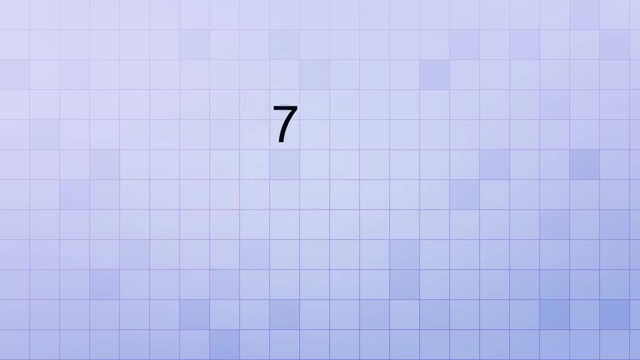 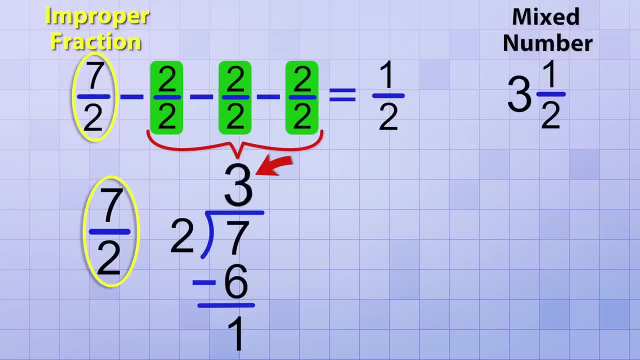 If we divide 7 by 2, we find out that 2 will divide into 7 three times, leaving a remainder of 1. to subtract out of the improper fraction 3.. So the answer to the division tells us what the whole number, part of the mixed number, will be. 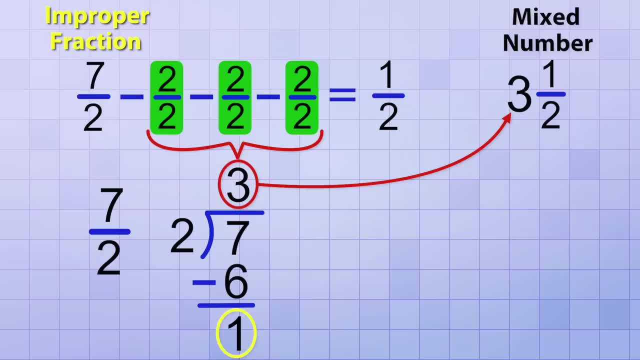 And here's the really cool part: The remainder of the division tells us what the leftover fraction will be. The remainder is the numerator of the leftover fraction. In this case, since the remainder is 1, we'll have 1 over 2 left over in our mixed number. 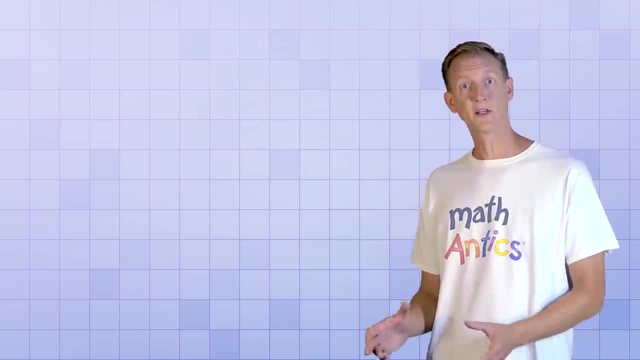 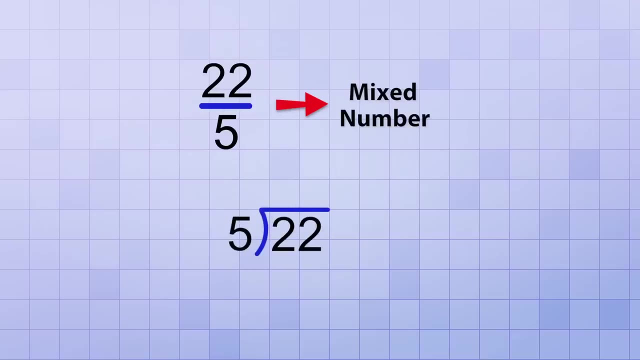 Let's do one more example to make sure you've got that. Let's convert 22 over 5 into a mixed number. If we divide 22 by 5, we see that 5 will go into 22 4 times, with a remainder of 2.. 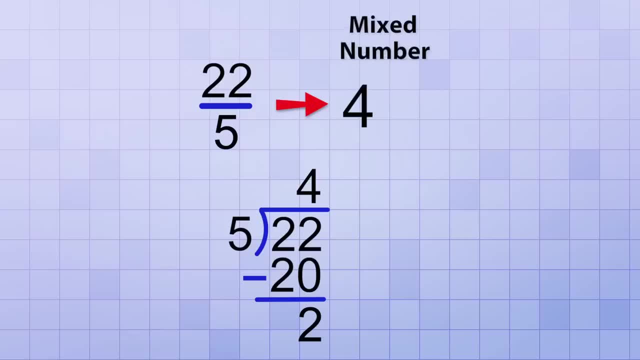 That means that the whole number part of the mixed number will be 4 and the fraction part will be 2 over 5, because our remainder was 2.. That's how many fifths will be left over. So 22 over 5 is the same as 4 and 2 fifths.